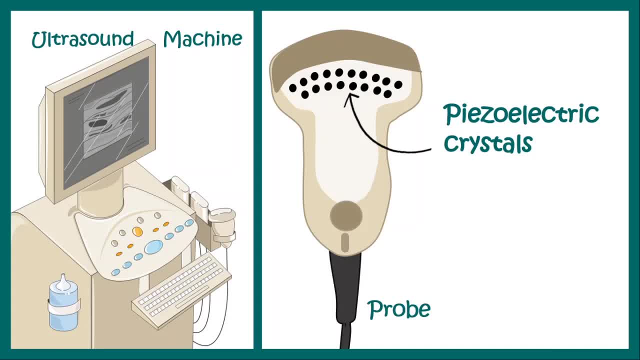 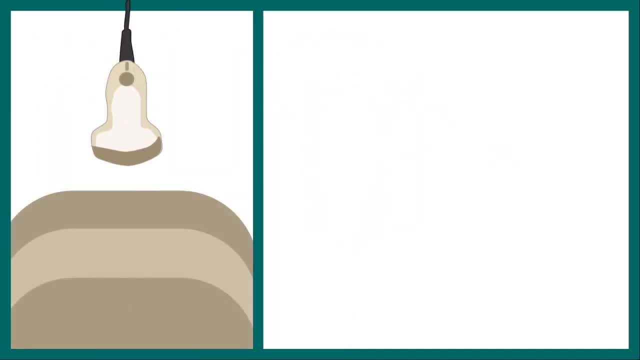 come to these piezoelectric crystals, they again produce electrical patterns. Now, when this probe is put over a body surface and supplied with electricity, the piezoelectric crystals generate sound wave. This sound wave gets reflected back to this probe, The piezoelectric 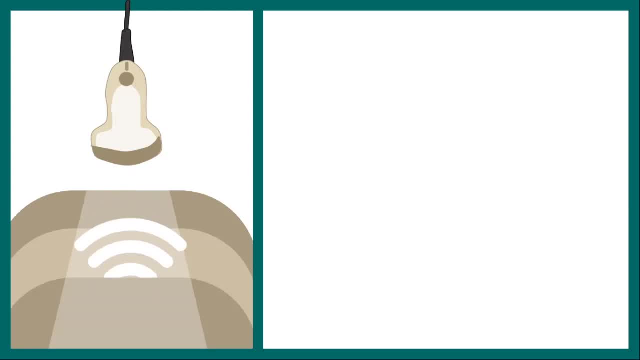 crystals sends this mechanical vibration and produce electrical pattern. Now ultrasound works due to the reflection of a beam at the boundary between the between two materials of different densities, because in human body different tissue have different densities. Now this electrical pattern that is generated by the piezoelectric crystals, 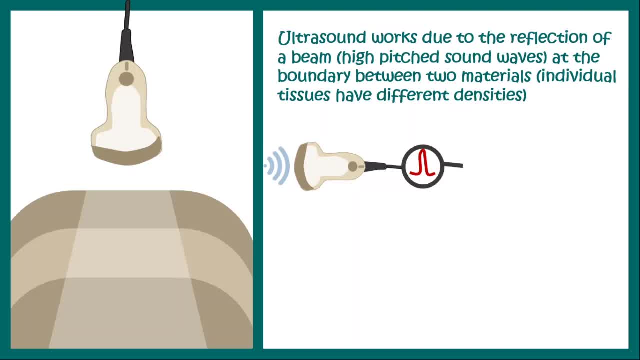 present in the probe in response to the mechanical vibration received back as a reflection from the tissues is analyzed by the software in a computer and a image is produced. Now this image is known as the ultrasonograph. Now the reflected wave is recorded and analyzed for its intensity. that 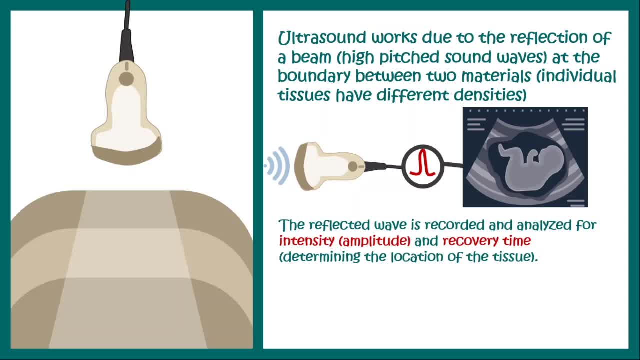 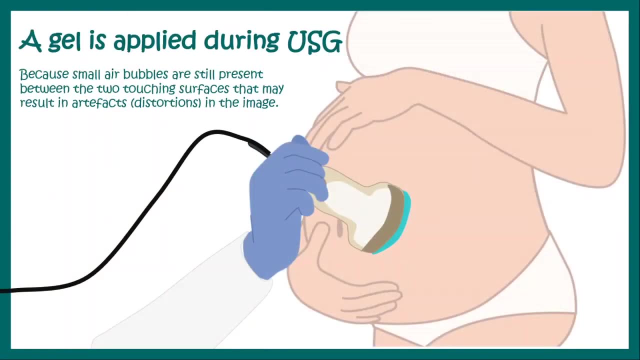 gives the amplitude and recovery time, which tells about the depth of different tissues and tissue layers and gives an idea about the location of the tissue. Now this allows us to assess the size, shape and structure of the organs and tissues. Now a gel is applied during USG and this is because 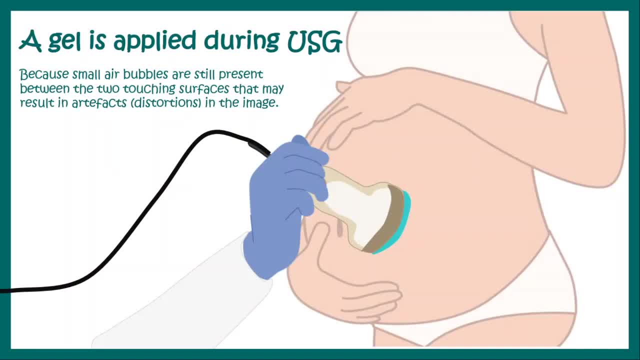 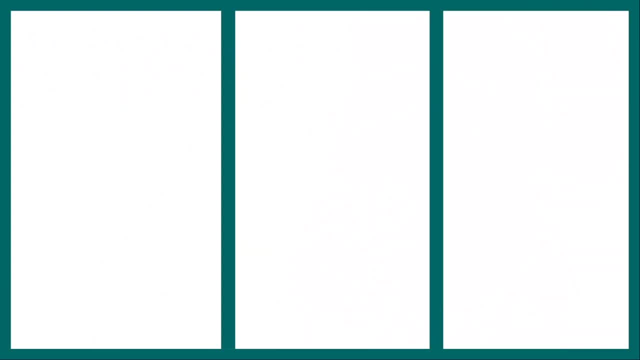 small air bubbles can be still present between the probe surface and the body surface, which can give rise to distortions in the image known as artifacts. Now there are different sort of probes used in USG, such as the curvilinear probe, linear probe or phased array probe. Different probes have different applications. Now let us 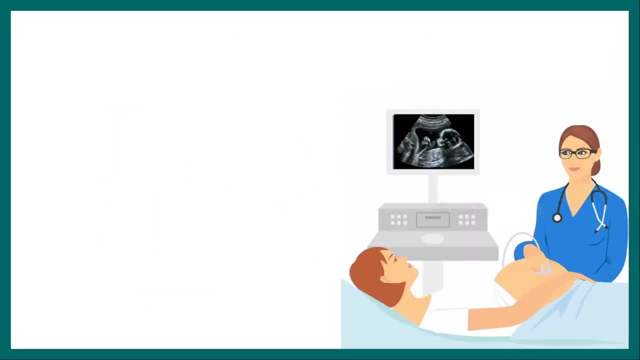 understand how we interpret USG images. Now, when we put a probe on the body surface, the part of the image near to the probe appears like this: Now this image appears like this: Now, when we put a probe on the body surface, the part of the image near to the probe appears like this: Now, this: 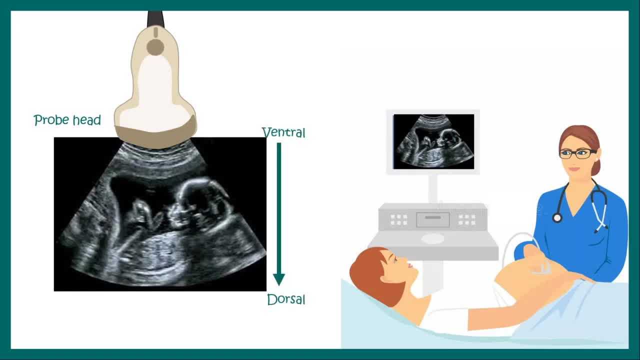 image of area of the image appears even narrower and the part away from the probe appears wider. Now, solid tissue, such as bone, will appear white orlahyperequake, because the outer surface reflects more sound wave or ultrasonic wave, Whereas the tissue that are filled with 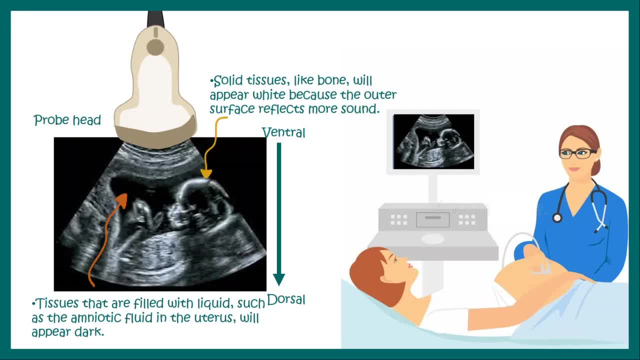 liquid, such as amniotic fluid in the uterus, runs on the bone surface. Now ultrasonography imaging does not work well for gas, So organs that are filled with air, like lungs, are generally not examined with ultrasound. There's a popular saying that goes in medical schools that air is the enemy of ultrasound. 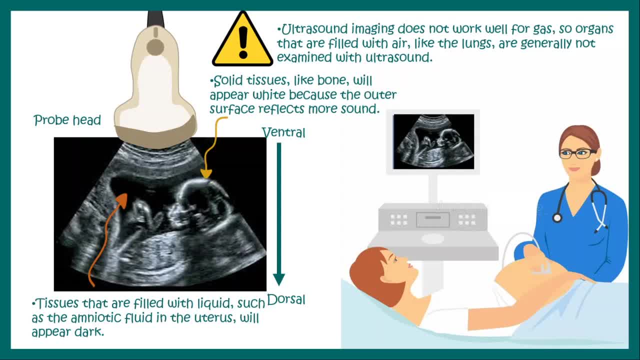 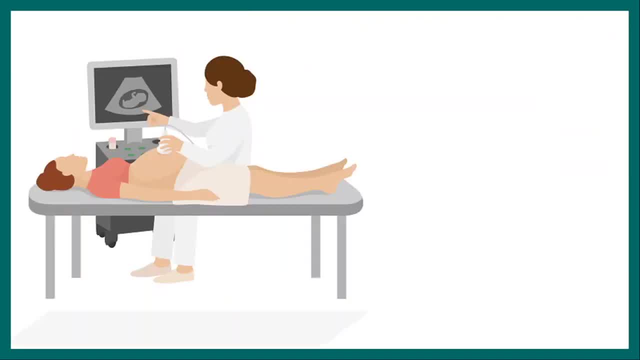 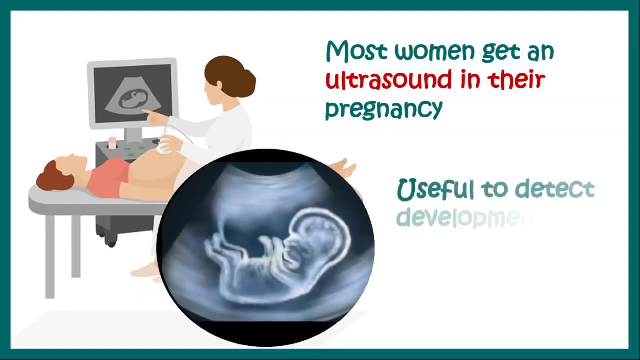 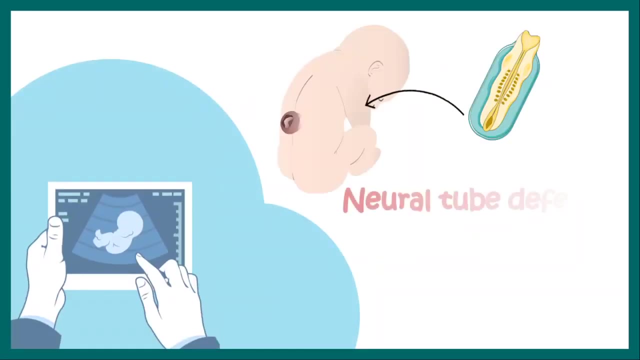 and fluid is friend and remember, ultrasonography does not use any radiation, So you don't have a risk of getting radiated. Now, ultrasonography is done in most women during their pregnancy. This imaging technique is useful to detect developmental defects. For example, ultrasonography is used to detect neural tube defects such as spina bifida. during 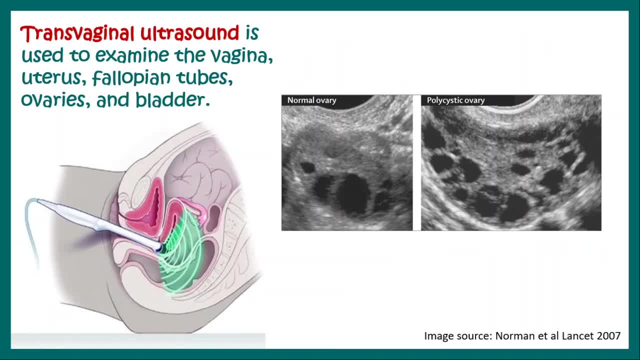 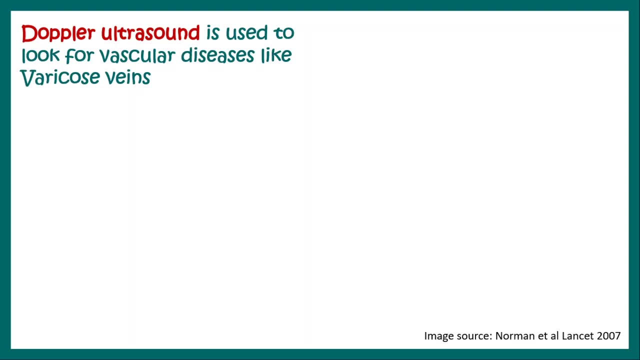 your pregnancy or transvaginal ultrasounds can be used to examine vagina, uterus, fallopian tubes, ovaries and the urinary bladder and is very routinely done by gynecologists. Other ultrasounds, Like Doppler ultrasound, is used to look for vascular diseases like varicose veins. 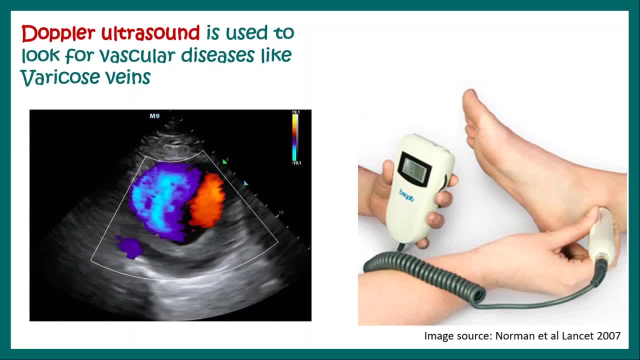 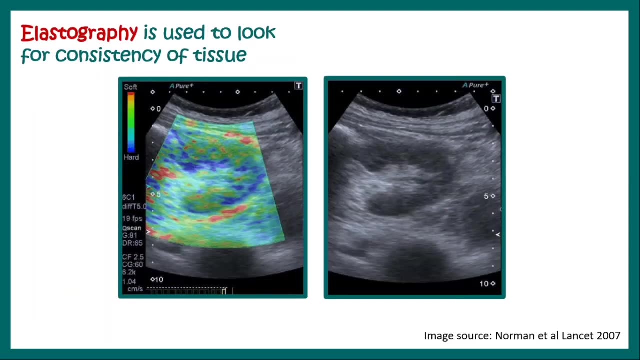 And this uses the principle of Doppler effect. in this ultrasound technique, And by using Doppler effect, they try to image the velocity and direction of flow of blood through the blood vessels. Again, another type of imaging that uses ultrasound is known as elastography, which uses different 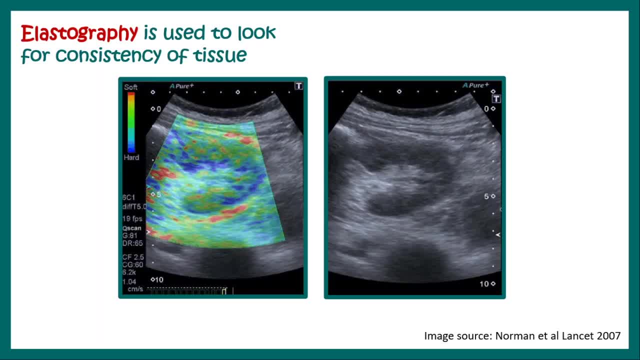 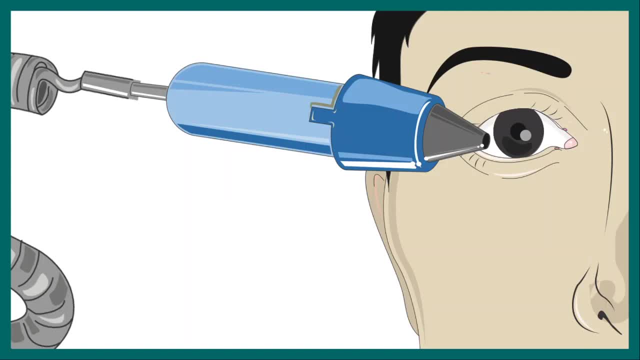 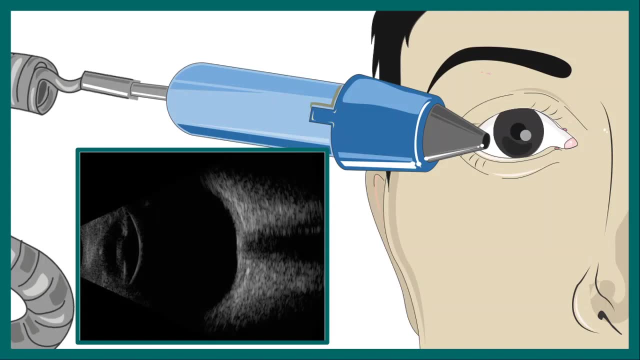 colors And represents the consistency of a particular tissue, as seen in this image. Now ultrasonography can be used to image eye and can detect different conditions of the eyeball. Now this image shows a normal eye USG and I believe you can make out the normal contour. 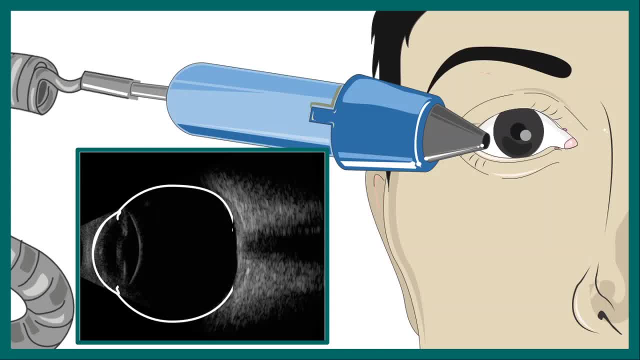 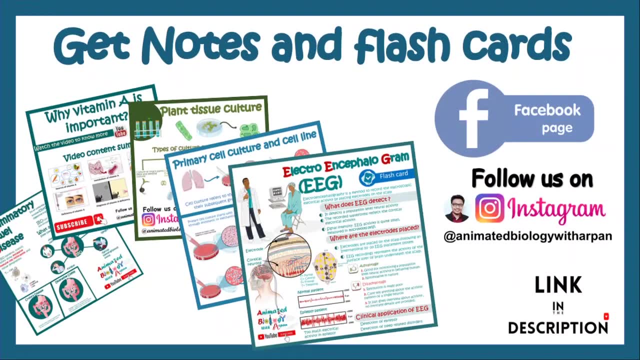 of the eye. So this is more or less the idea about ultrasonography or USG. If you have enjoyed this video, please do hit the like button. Share this video, Share it with your friends and peers And do subscribe to the channel. 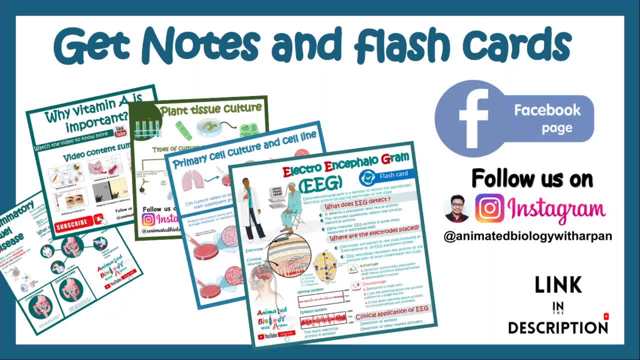 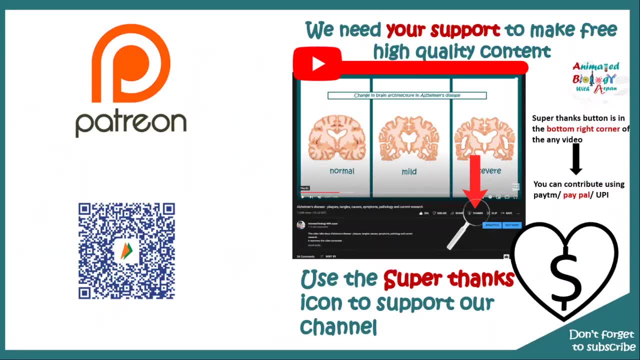 To get high quality notes and flashcard. follow the Facebook page and Instagram of Animated Biology with Arpan. The link will be in the description box. Also, we need your support to make high quality content on this channel, So support us on Patreon. or also you can use the super thanks button in the bottom right. 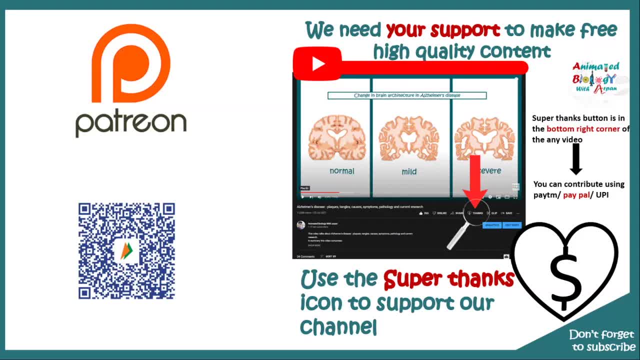 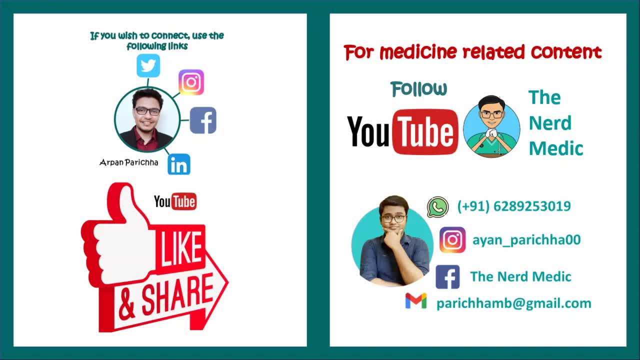 corner of the video and can contribute using Paytm, Paypal or UPI. Again, If you wish to connect with Arpan Pareecha of Animated Biologist with Arpan, the links will be given in the description box And for medicine related content, you can subscribe to my channel, The Nerd Medic on. 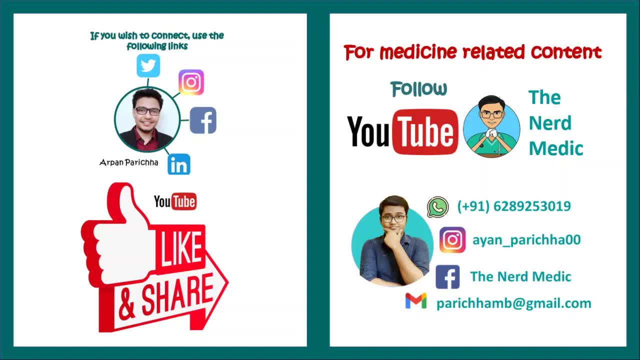 YouTube Also. if you want to get in touch, you can connect me via WhatsApp, Instagram, Facebook or email. The IDs are given on the screen. Until then, bye, bye, See you in the next video. 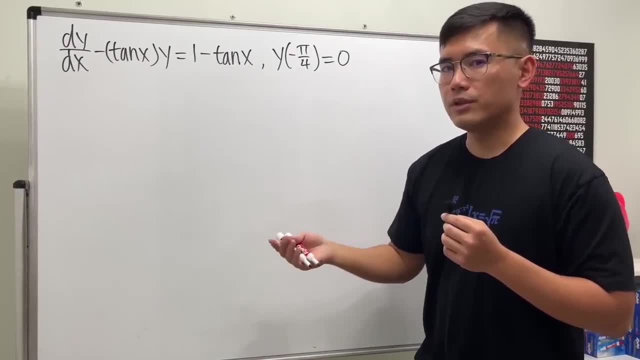 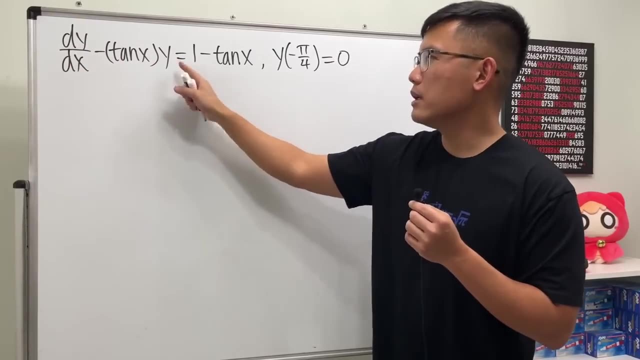 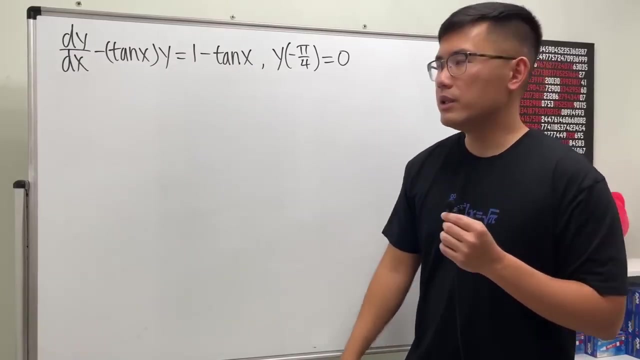 And now this one is actually very different than the previous two because this is not separable. Have a look: We have dy, dx minus tangent x, and then multiply by y, So the y is not itself the tangent, And then this is equal to 1 minus tangent x. This is called the first order. 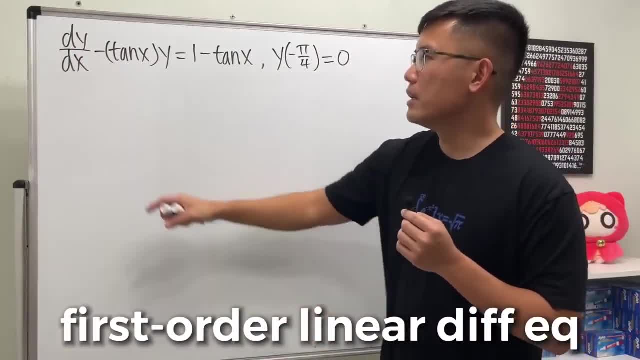 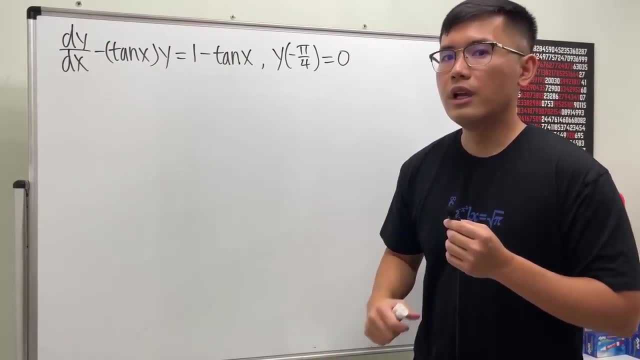 because we have the first derivative, Linear, because all the derivatives and also the y's are of the first power, First order linear differential equation. And the way that we're going to handle this is that we'll use the so-called integrating factor. I have a video. 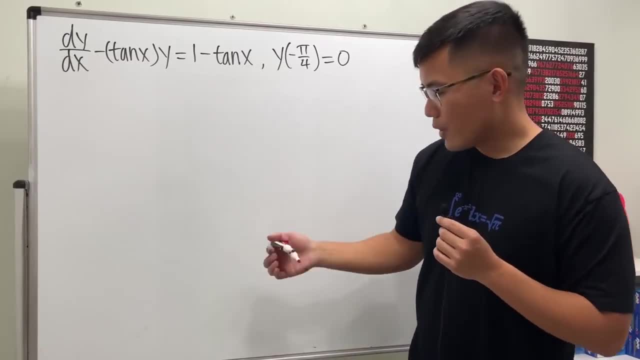 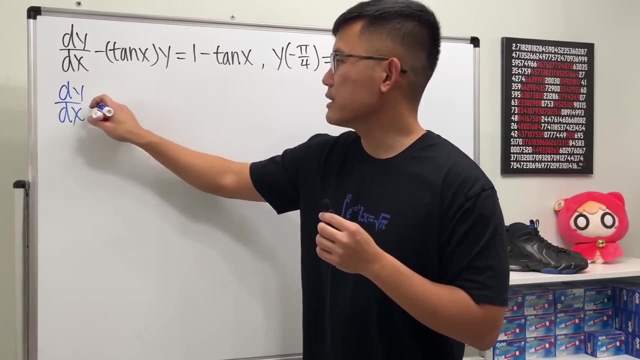 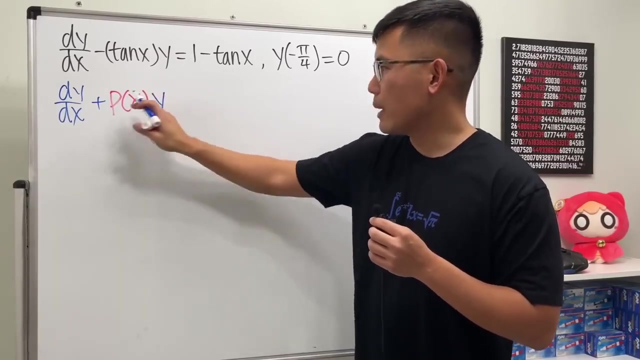 on that already. You guys can go ahead and check that out, So I will write that down for you guys, though what it is. We must have the equation in the standard form, namely dy, dx plus some function in terms of x. So let's call that p of x and then multiply by y And 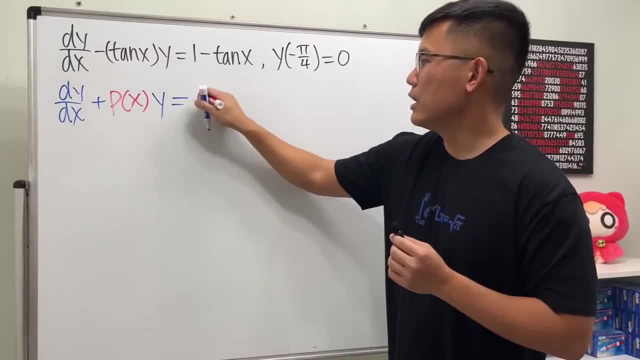 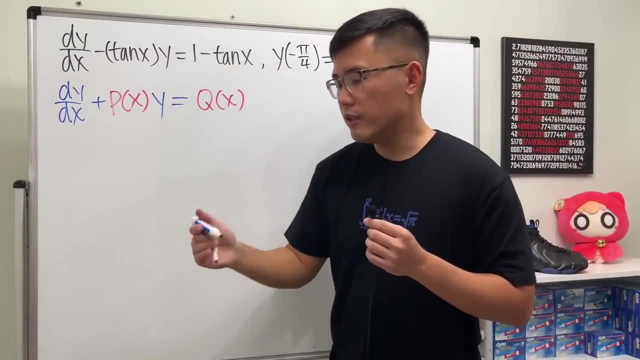 anyway, we have the first order linear differential equation And the way that we're going to handle anything else in terms of just x, you will be on the right hand side, So notice that this right here does not have the y, So it fits this category. Now the integrating factor, abbreviated as i, f.